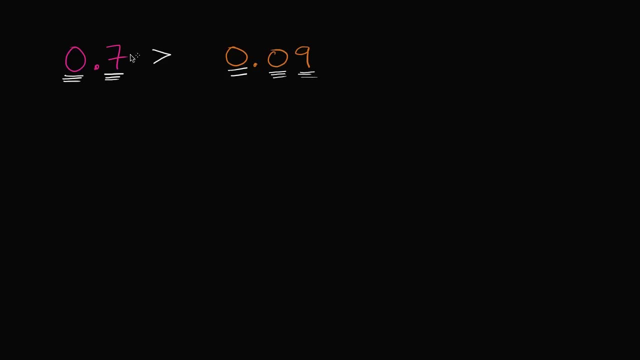 to the right: you have nine hundredths here and you have no hundredths over here. We could write a zero over here and you'd say: oh well, look, you have no hundredths over here, But the nine hundredths don't matter. 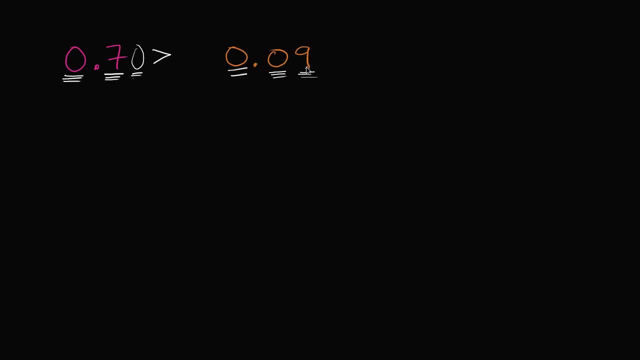 Remember, even if you had ten hundredths, that's the same thing as one tenth. So it doesn't matter that nine is somehow greater than seven. What matters is it's in a place to the right, Even if you increased by another hundredth here. 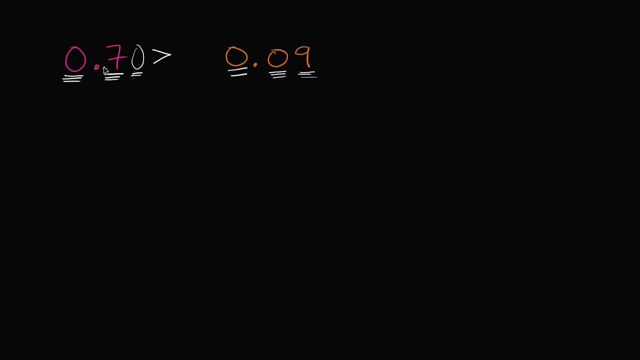 you'd only get to one tenth. This thing over here has seven tenths. Let's do another one of these. Let's say: let's say we wanted to compare. let's say we wanted to compare 0.0.29,. 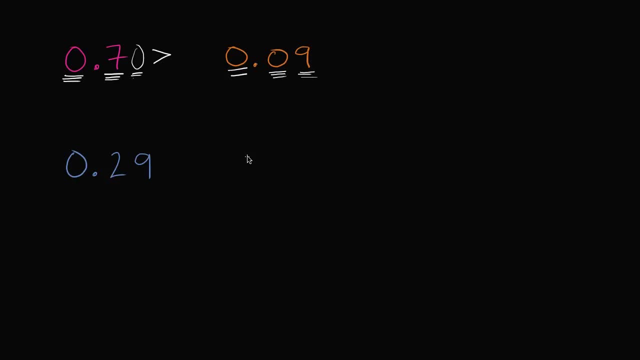 and I want to compare. let's say, I want to compare that to 0.31.. Now this one, you might say, is a little bit more straightforward, depending on how you think about it, If you say, hey, this is 29 hundredths. 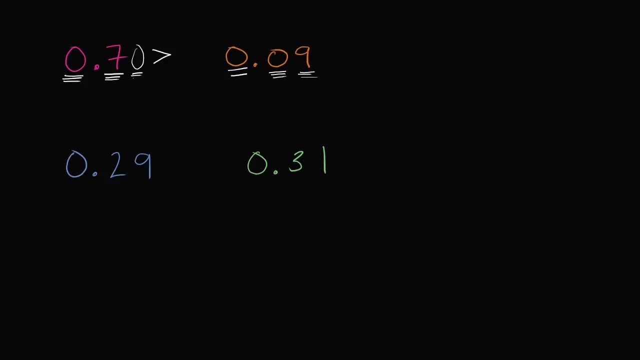 this is 31 hundredths. wait, I have more hundredths on the right hand side. So let me open my inequality to the larger value and I would say: 0.29, or 29 hundredths is less than 31 hundredths. 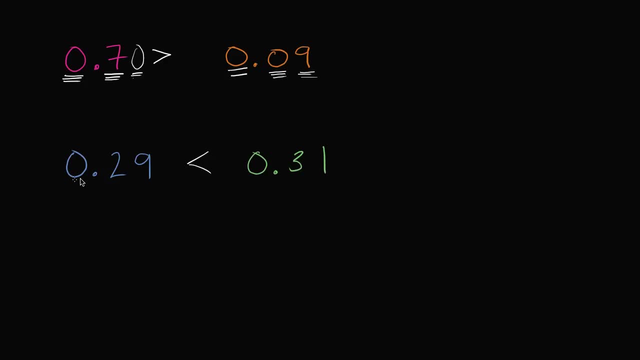 Another way you could have done this is you could have looked in the ones place, Say, okay, they both have zero ones, But then you look in the tenths place, say this only has two tenths. well, this has three tenths. 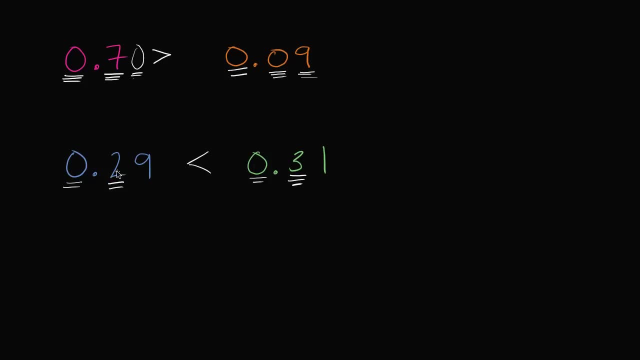 I actually don't have to keep looking at the digits to the right of that. I could just compare this two tenths to the three tenths. Three tenths is larger, And so I would say that 29 hundredths is less than 31 hundredths. 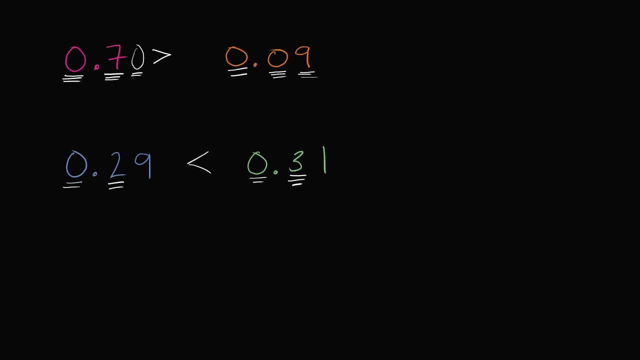 Let's do one more, just for fun. Let's compare. let's compare 0.6 to. I'll do them the same color, 0.06.. Which of these is the larger number? Well, we do the same thing that we've been doing. 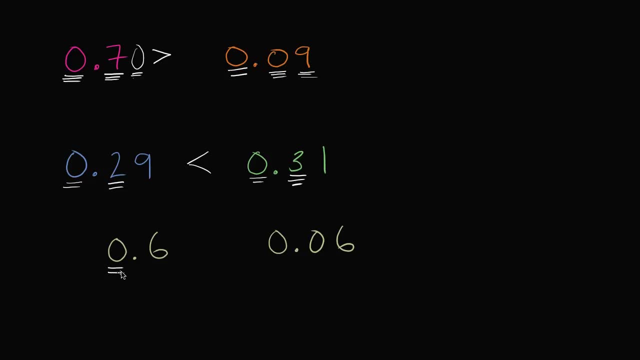 You can first go to the ones place, Say, okay, this has no ones, this has no ones, Okay, that doesn't tell us much. Then the tenths place: this has six tenths, This has zero tenths, So this number is going to be larger.